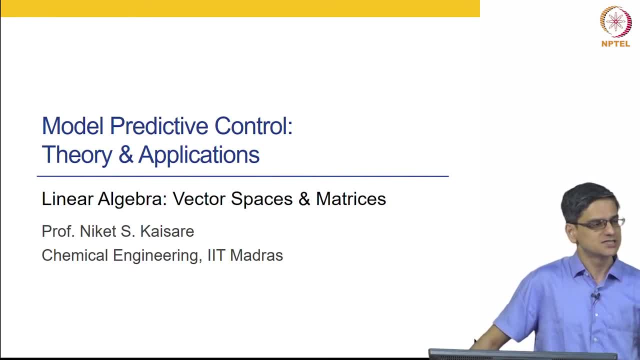 idea: ah, over here, And so it is. it is the same concepts that you have learnt. ah, mostly the. maybe a couple of them might be new, but mostly it is the same concepts that you have learnt, but we are going to do that in a way that is more. 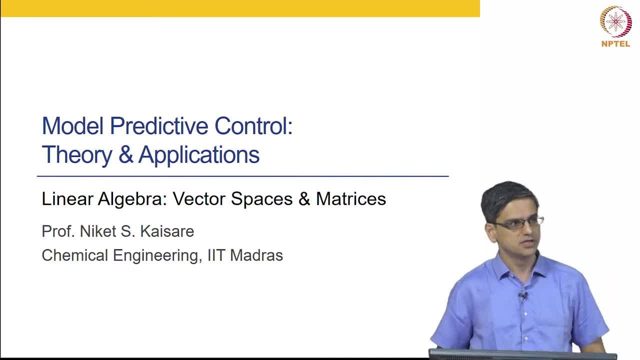 conducive ah to ah, the linear control systems, kind of a framework where ah, for example, if output y equal to a multiplied by u, then the matrix a is a matrix that does linear transformation. So we will get to that ah in tomorrow's lecture, but before that ah, 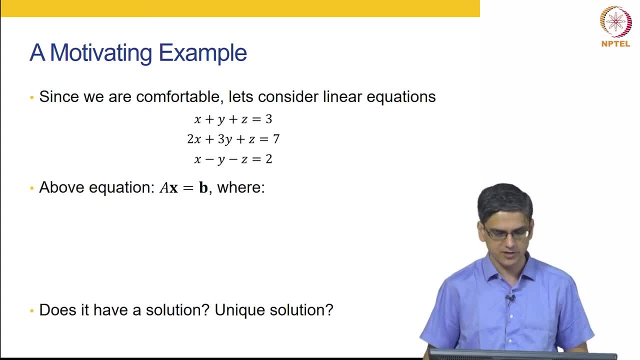 you know, let us, ah, you know, get. Let us start with what everyone, I am sure, is comfortable with. ok, ah, So let us say you are given this particular problem right. So we want to write this above equation in terms of a: x equal to b. How do you do that? You write this in terms of 1, 1, 1, 2, 3, 1, 1 minus. 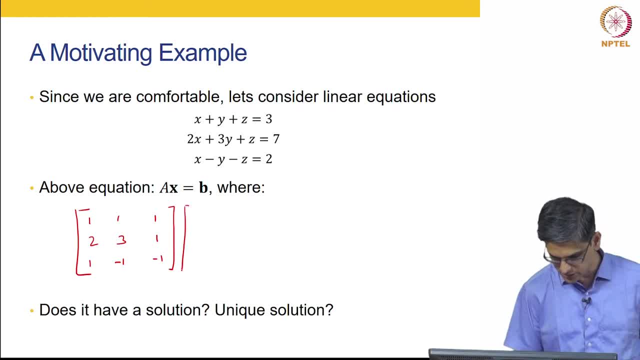 1 minus 1, multiplied by x, y z. 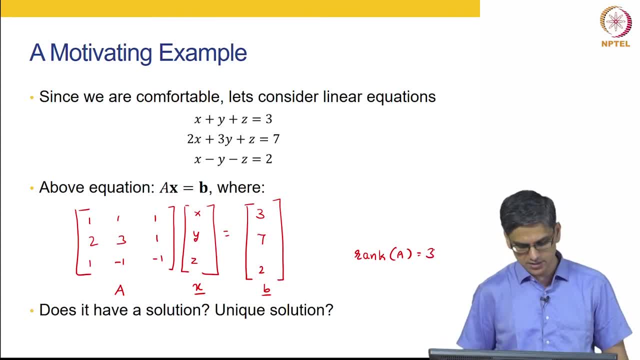 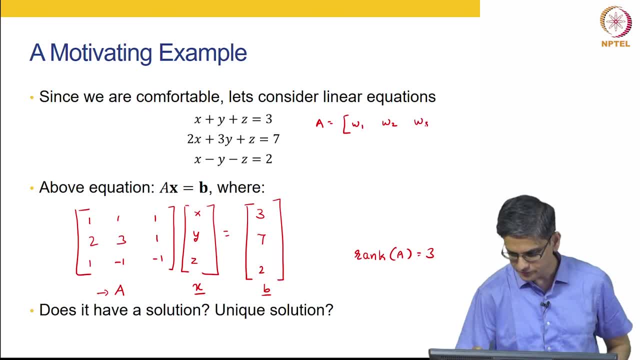 So ok, so this is w 1 bar, this is w 2 bar and this is w 3 bar. ok, and the matrix multiplication of A multiplied by x, y and z is nothing but x multiplied by w 1 bar plus y multiplied. 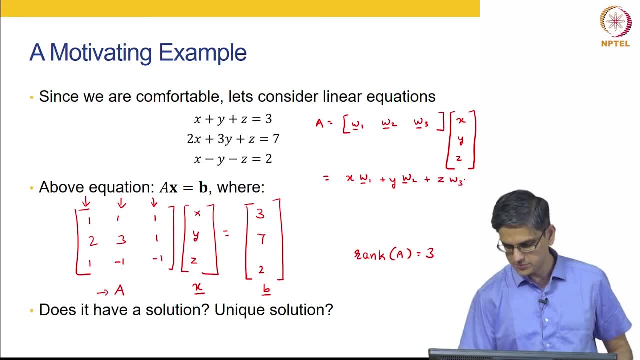 by w 2 bar plus z multiplied by w 3 bar. ok, So if this is A, then this guy is equal to this. ok, So the problem that you have dealt with so far, that is solving linear equations. we are just posing it in a slightly different context. we are writing the matrix A as 3. 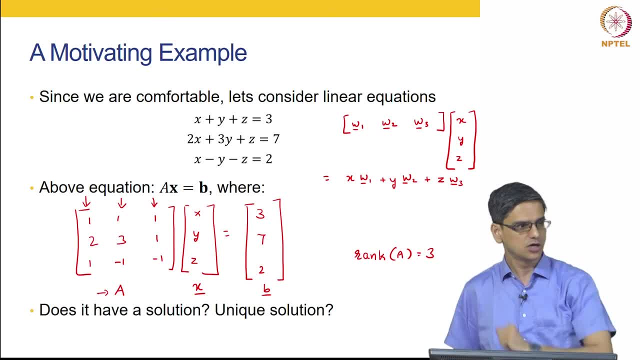 column vectors, Ok, Concatenated together, and that is multiplied with your vector x, bar and this particular thing you might recognize. this is nothing but linear combination of vectors w 1,, w 2 and w 3, or it is a linear combination of column vectors of matrix A. 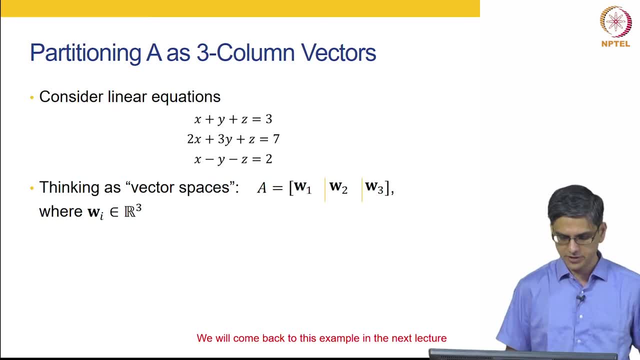 Ok, Yeah, So that is what we have written over here. So we are going to talk in terms of vector spaces. So b bar cannot be expressed as linear combination of vector spaces. Ok, Ok, So we are going to write bust operand in vector space. b bar can be expressed as center. 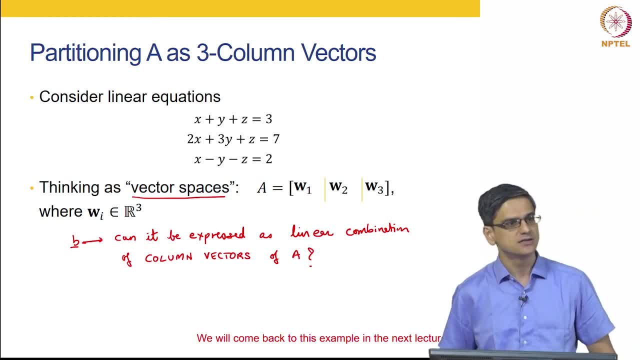 hijos of rounded aç column vectors of A. If the answer to this is yes, then a solution x, y, z exist. If the answer to this is no, then a solution x, y, z does not exist. Ok, It is possible that the matrix A has rank of 2 and still solution to Ax equal to b exists. 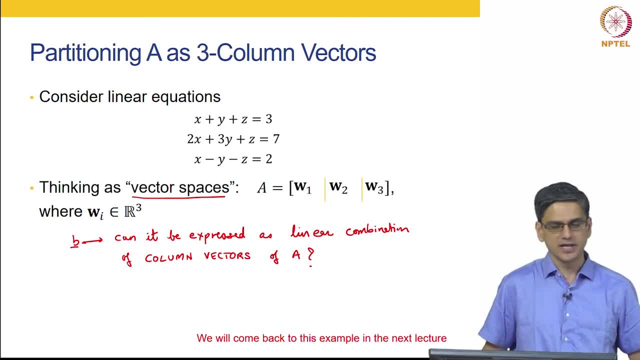 ok, That is the case when you have rank of A and rank of A, comma, B as the same. that is something that you have. you have studied. What that really means is that the matrix B can be expressed as a linear combination of the column vectors W1,, W2, W3, and the linear combination of these column vectors constitutes: